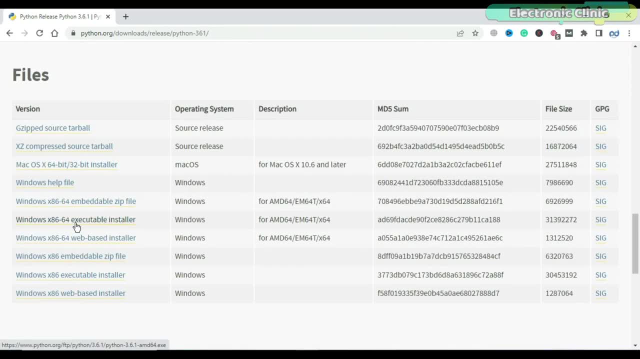 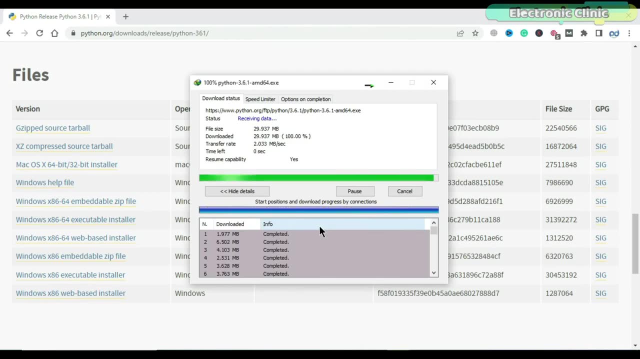 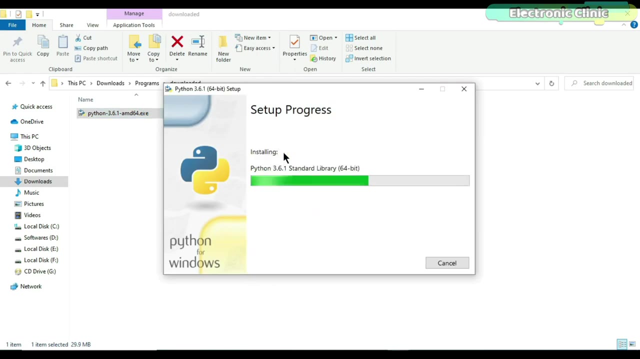 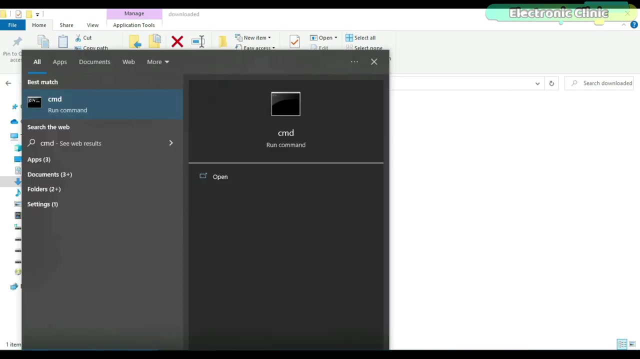 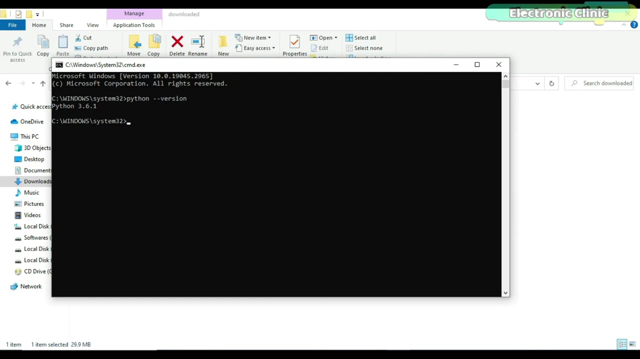 browser, Scroll down and download the Windows x86-64 executable installer. Double click to install the Python and make sure you check this box Now to check if the Python is installed, simply open the CMD Type Python double dash version. As you can see, Python 3.6.1 has been installed. 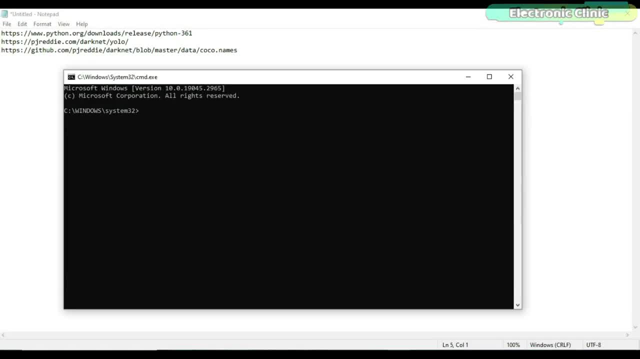 Next we are going to install OpenCV. Open the CMD command prompt and type this command. As you can see, I have already installed it. There is nothing complicated, It's just a simple installation process. Now we will install YOLO for this. Copy this link, Paste it in the. 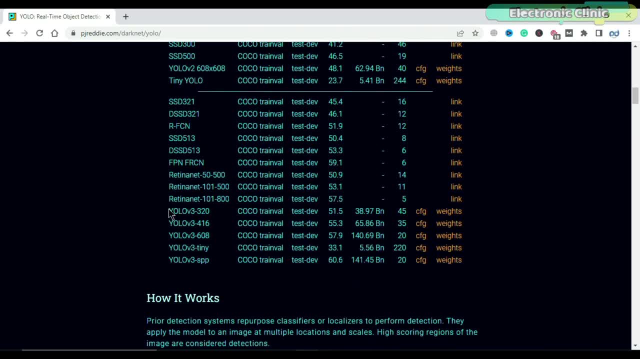 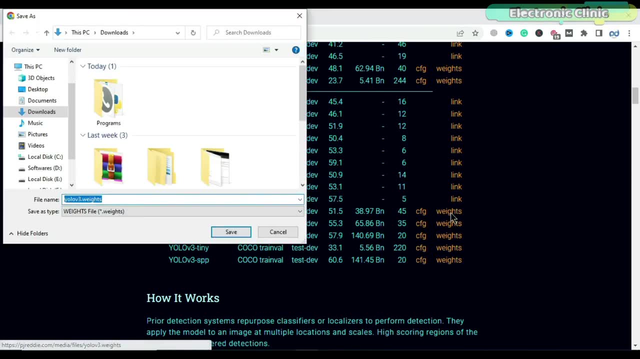 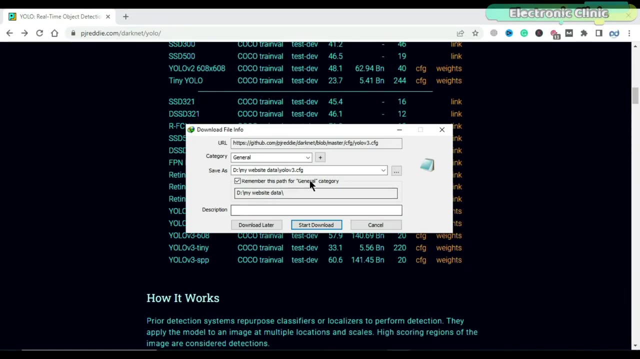 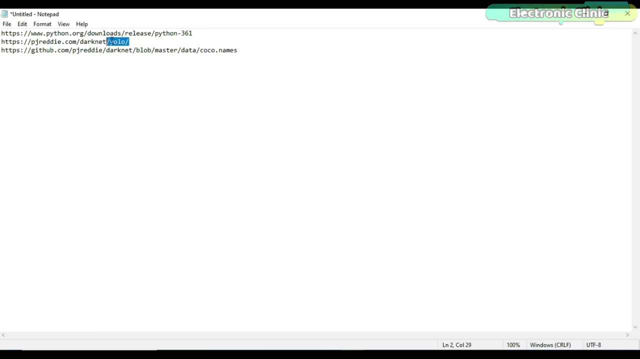 browser. Scroll down and download the weights and cfg files of the YOLO v3-320.. After downloading the weights and cfg files, next we will copy the coco dart names For this. copy this link and paste it in the browser. 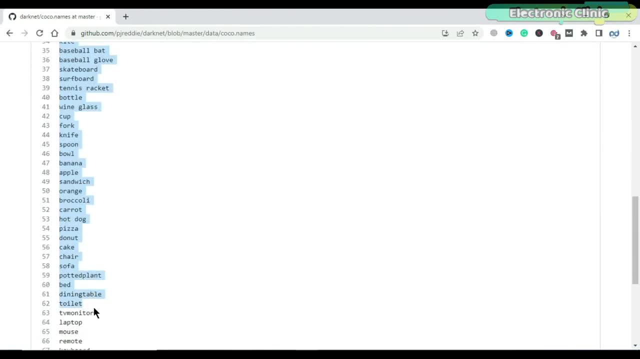 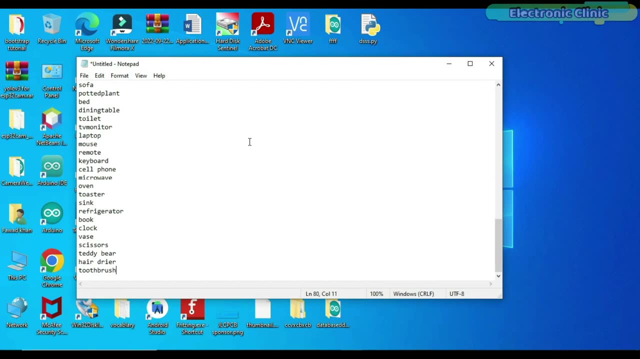 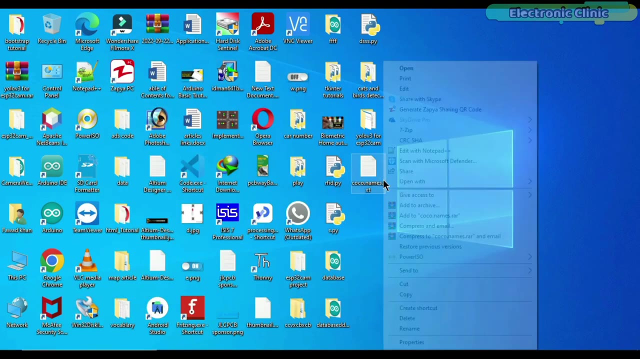 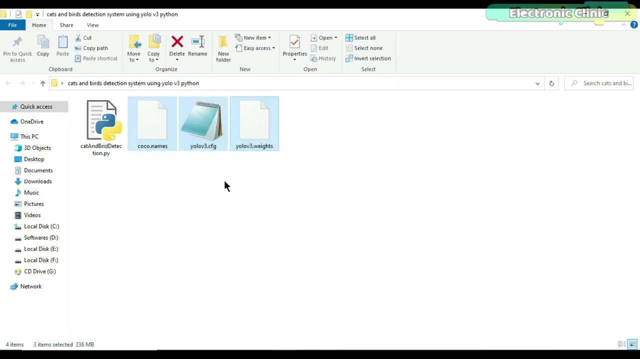 Copy all the names. Open notepad and paste these names. Save it with the name coconames. Remove the dart txt extension. Keep the coconames yolo- v3.cfg and yolo- v3.weights files in the same folder with the main programming file. The gate in bird detectionpy is the main programming file. 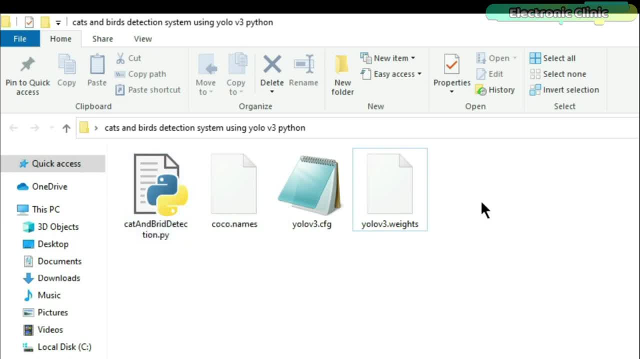 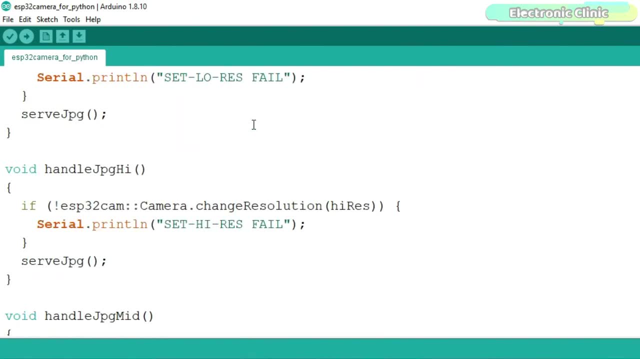 Next we are going to start with the ESP32 camera module. You will need to upload this program in to esp32 rumors module for the live video streaming. You can download this code from our website, electronicscliniccom. But first you will need to download this library. But 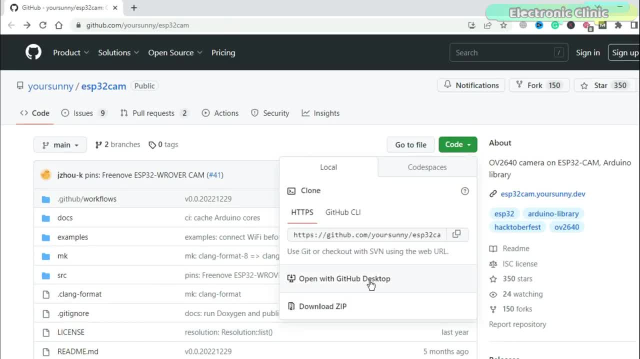 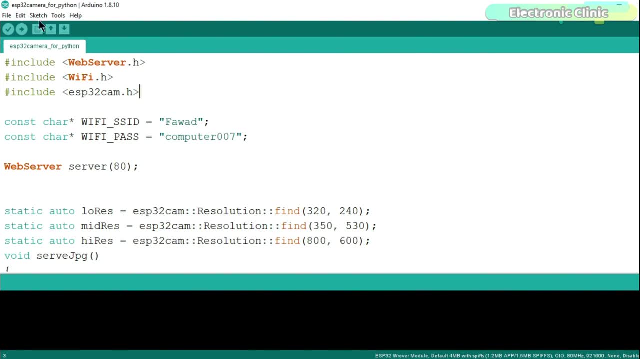 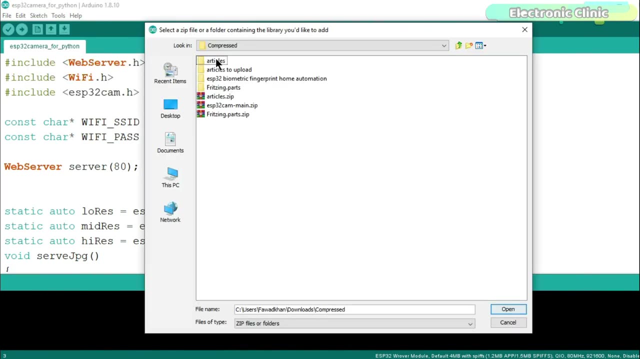 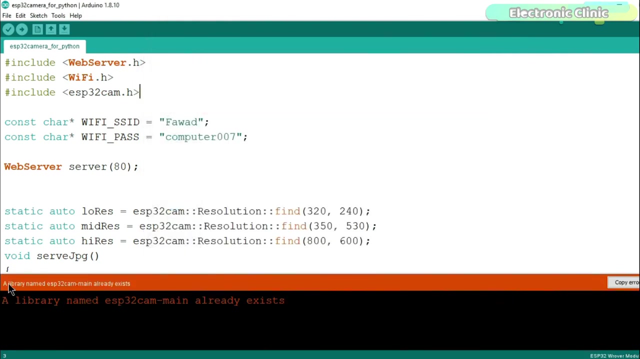 this is going to get up and download the ESP32 GAME zip. Then go back to Arduino IDE, Click form the sketch menu, Then include library And click on the azip libraryNewenerZIPine instance file. Then browse to the location and select the zip folder. As you can see, I have already added this library For 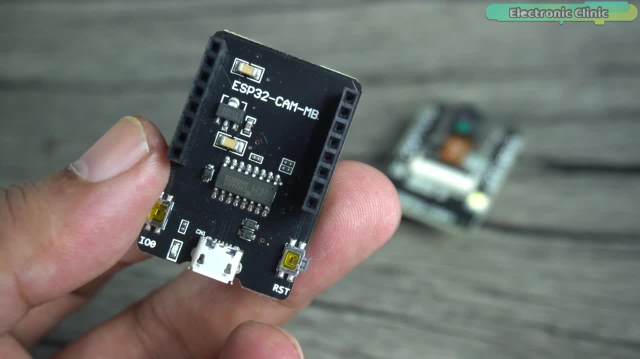 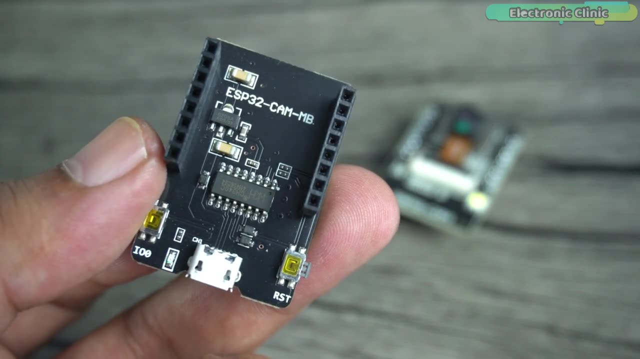 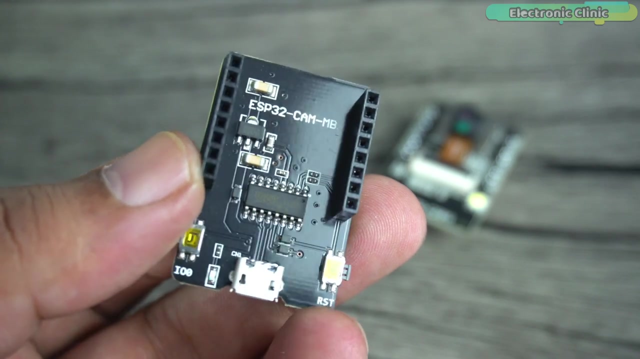 uploading the program. I'm using the ESP32 camera development board. This way, I don't need to use Arduino. but if you don't have this development board, then you can use the Arduino Uno for uploading the program. For this, you can watch my getting started video on the ESP32 camera module: Simply insert the. 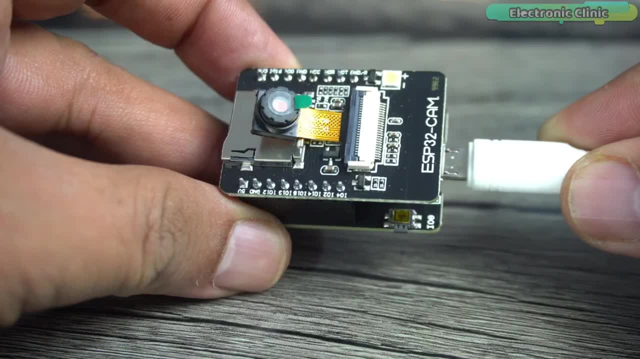 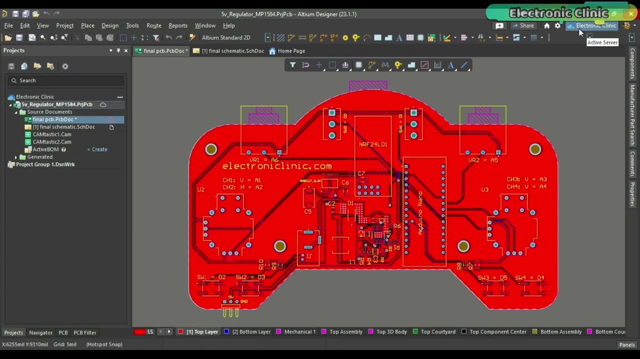 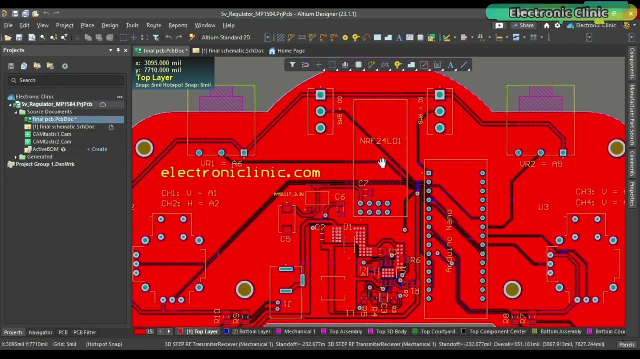 ESP32 camera module into the development board and connect it to your laptop or computer. Get your Altium 365 workspace activated, because Altium 365 provides a useful solution in cases when you are facing difficulties with your PCB design and unsure of your next step. You can share your project in Altium. 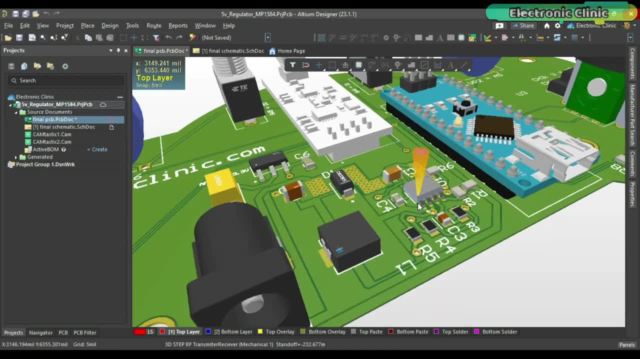 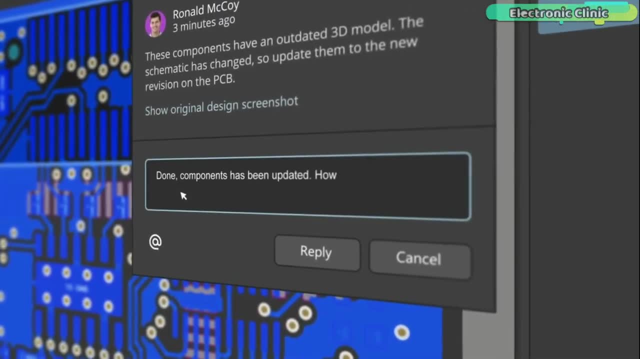 designer or on the web with any user. in just a few clicks, You will have full control over who you want to connect to, Who you want to give read-only access for, let's say, comments and design inspections, and who you want to give read-write access to allow full global. 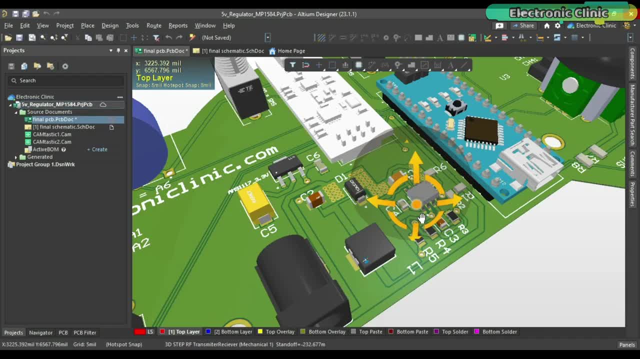 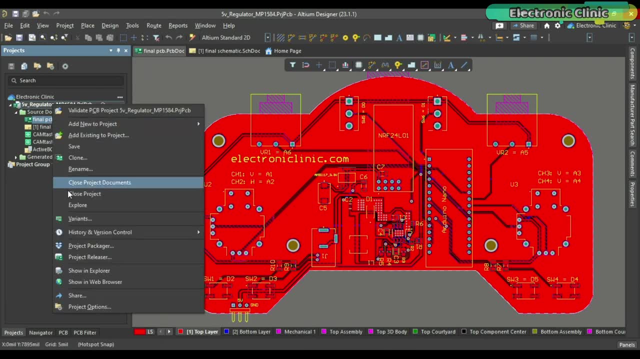 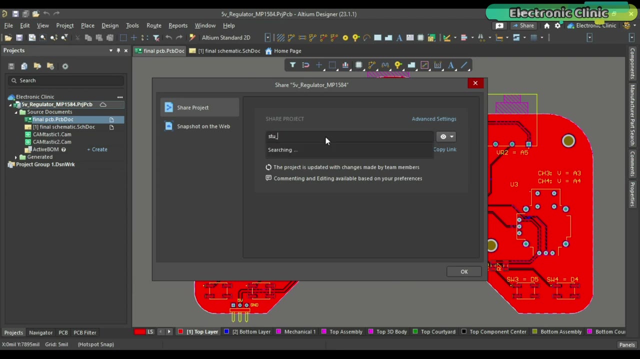 collaboration by a geographically dispersed team, with editing performed through Altium designer. Let me show you how to share your project. Simply right-click on the project name and select share. Write the user's email. Select read or write permissions from the drop down menu on the right. 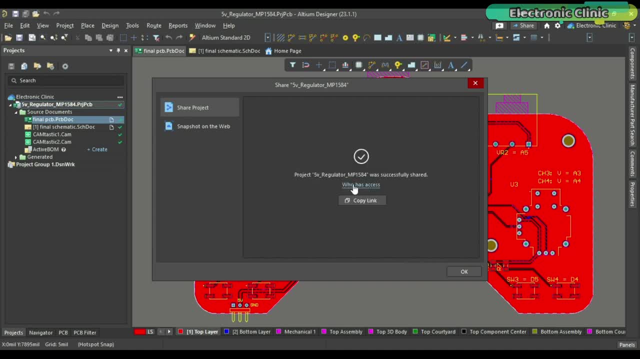 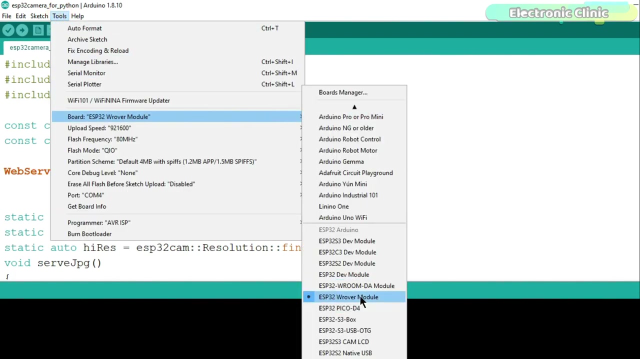 and click on the share button. It's just that simple. I've added links to the Altium designer, Altium 365 and Octapod, the world's fastest component search engine. Now let's get back to our project. Select the ESP32 game board, then check. 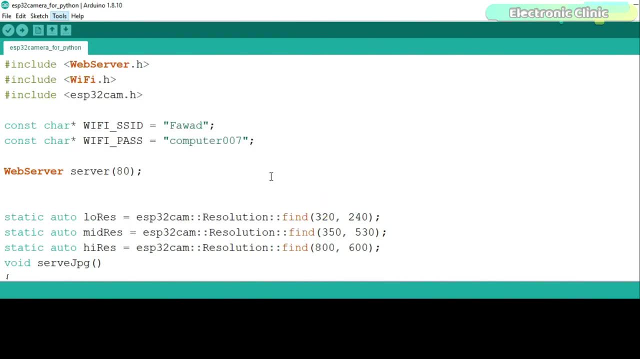 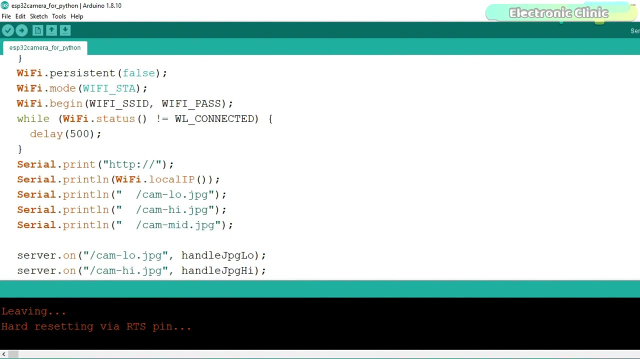 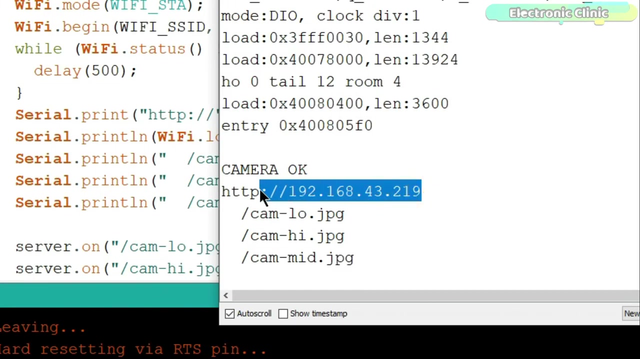 the communication port and then finally click on the upload button. You can see the program has been uploaded. After uploading the program, restart your ESP32 camera module. Then open the serial monitor. Wait for the ESP32 camera module to connect. Copy this IP address. 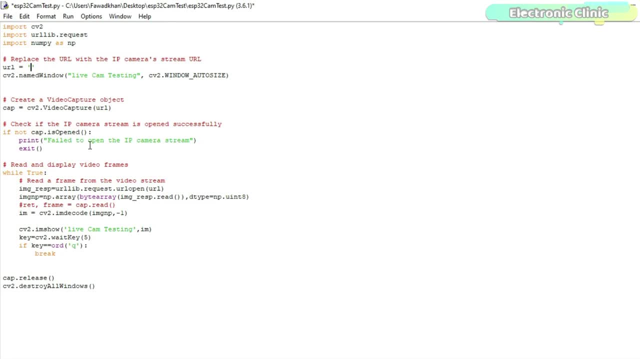 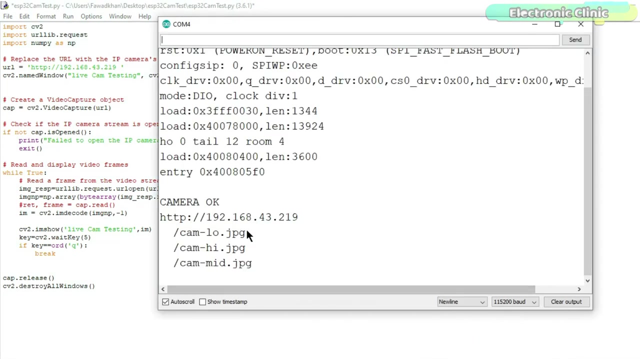 You will need this Python OpenCV code. You can download it from our website, electroniccliniccom. Paste this IP address Again. go back to serial monitor. You can see we have three different image resolutions: low, high and mid. Use the one as per your needs, but I'm going to start with low resolution. 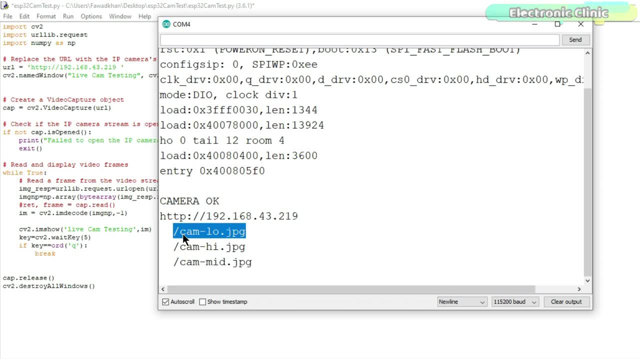 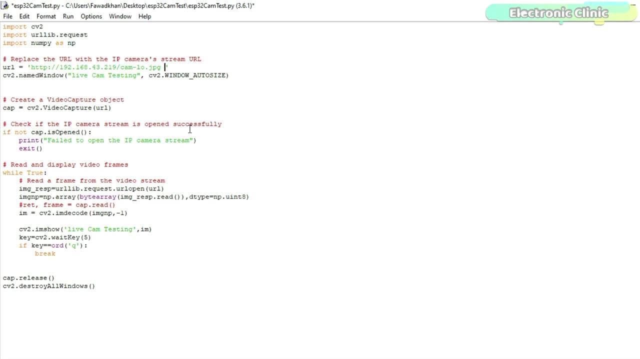 You can see we have three different image resolutions: low, high and mid. Use the one as per your needs, but I'm going to start with low resolution. You can see that there isn't any volume at all. Paste it next to the IP address and make sure there are no spaces. otherwise 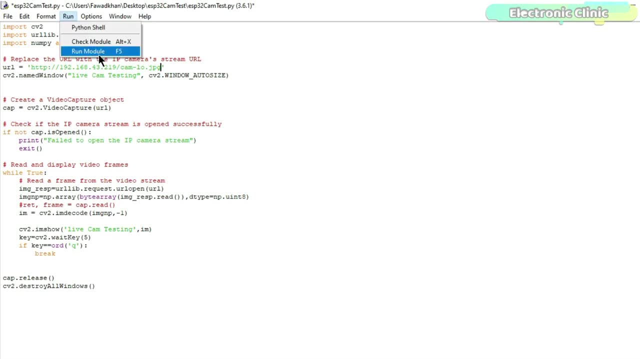 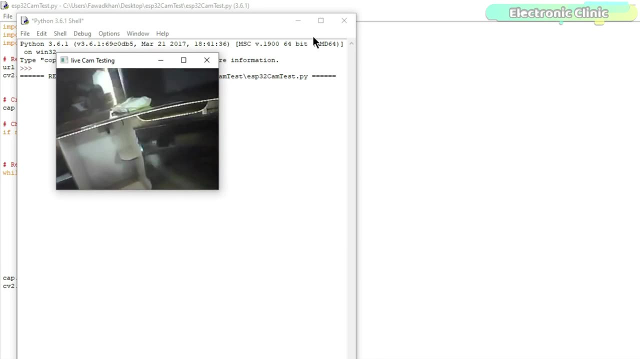 it will give you an error. Remove the extra spaces and run the program. As you can see, we can do the live video streaming, but as I'm using low image resolution, that's why the image isn't good. Let's try high image resolution. 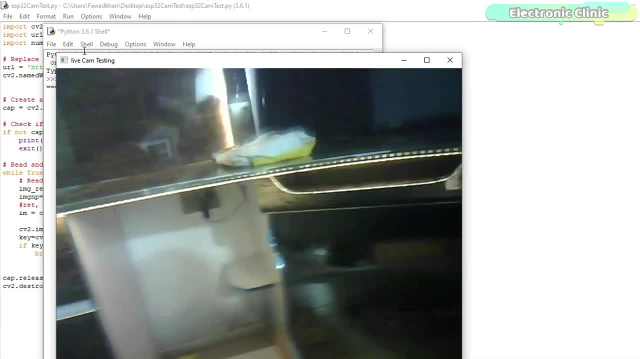 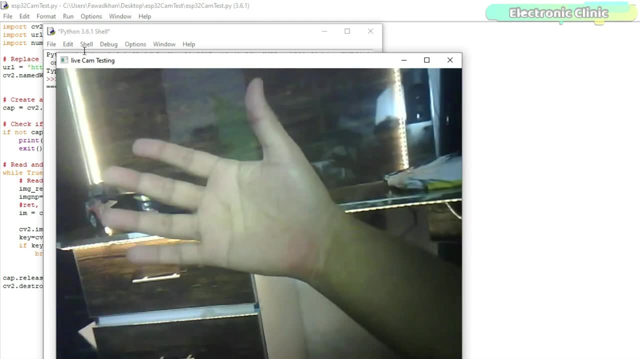 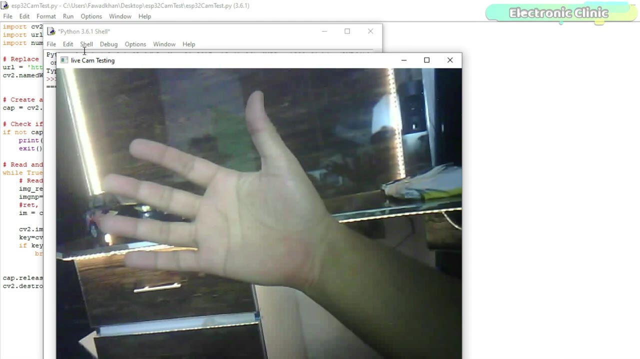 It's working. so the ESP32 camera module is ready for the object detection and identification using YOLOv3.. Let me tell you we are only using ESP32 camera module for the live video streaming. We are not doing image processing on the ESP32 camera module. 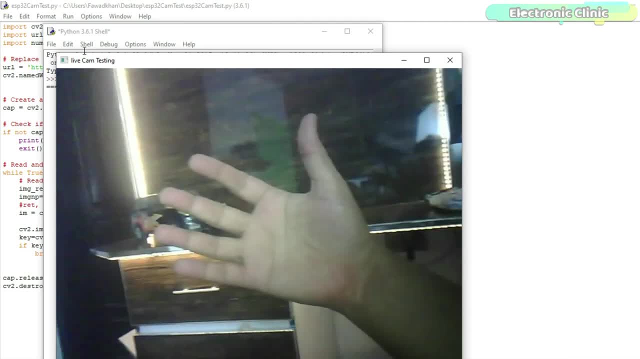 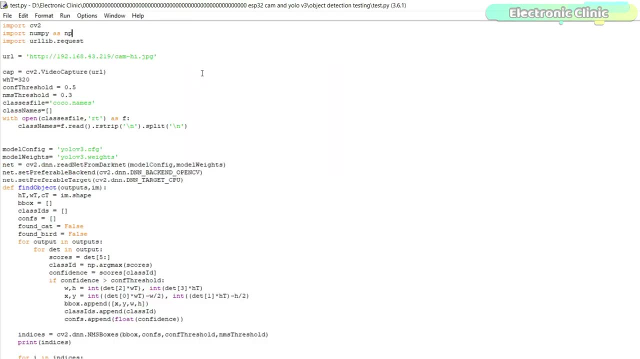 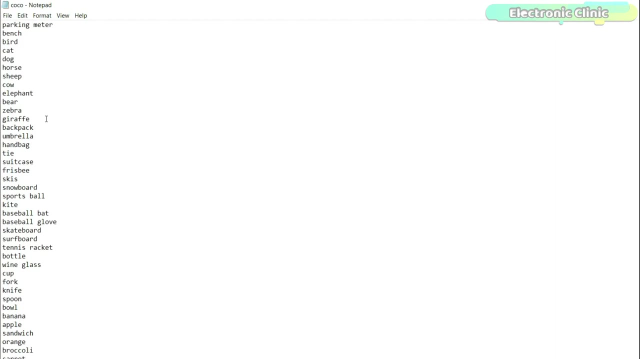 The image processing, object detection and identification will be done on a laptop or Raspberry Pi, So let's go ahead and do it. So first, let's go ahead and check this test code written for the detection of all the objects. By all objects, I mean only those objects which are available in the coconames list. 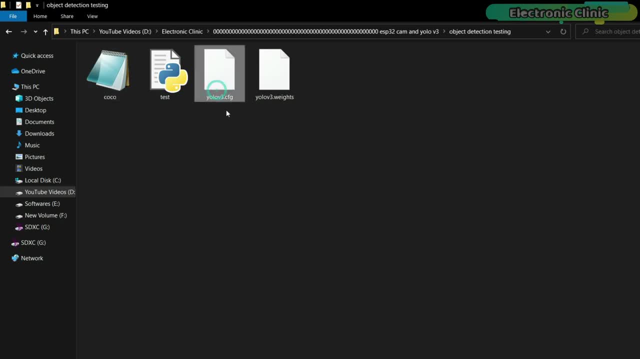 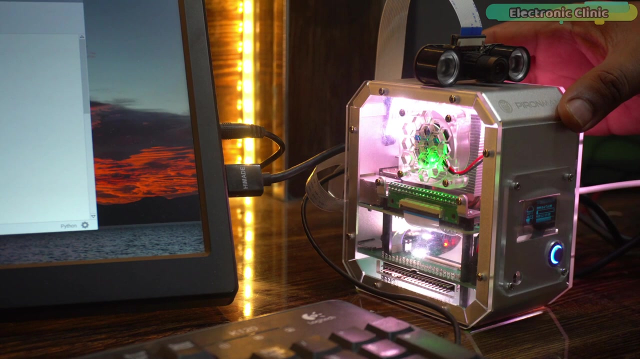 And make sure you keep the coconames, YOLOv3.cfg and YOLOv3.waits file in the same folder with the main programming file. So first let's start with the Raspberry Pi. So, guys, this is the smallest Raspberry Pi for PC and it has 8GB RAM. 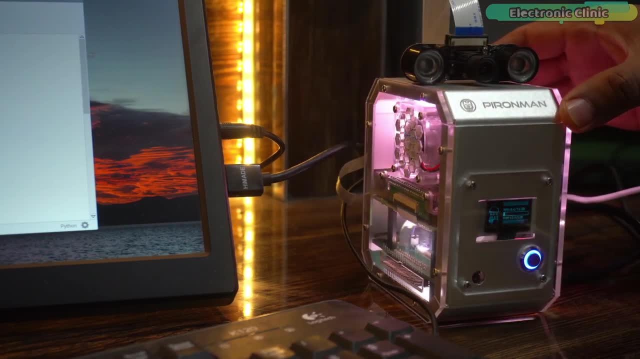 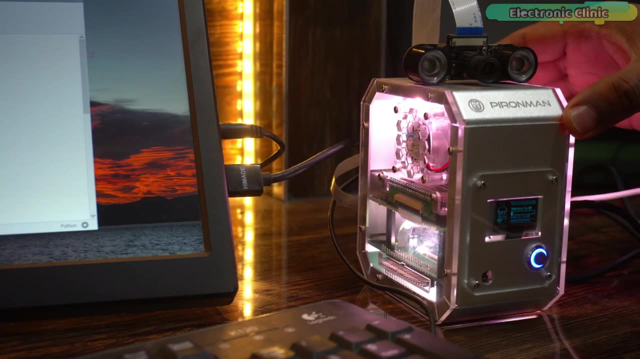 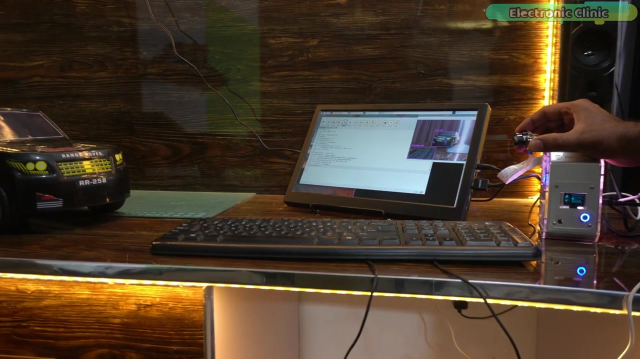 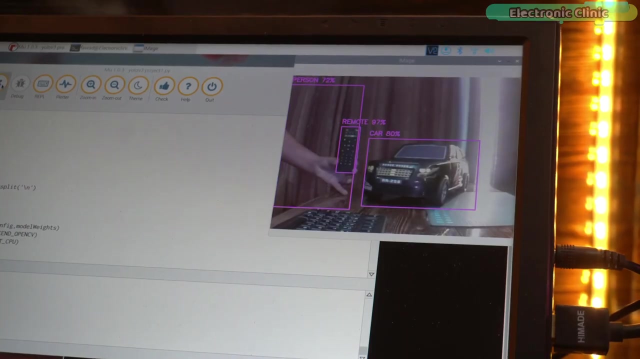 I got it for $10.. I got it from SunFounder. The reason I am doing this test is just to let you know that is it powerful enough to handle image processing using Python, OpenCV, YOLOv3.. I already have a camera connected to my Raspberry Pi, so I am going to use this camera. 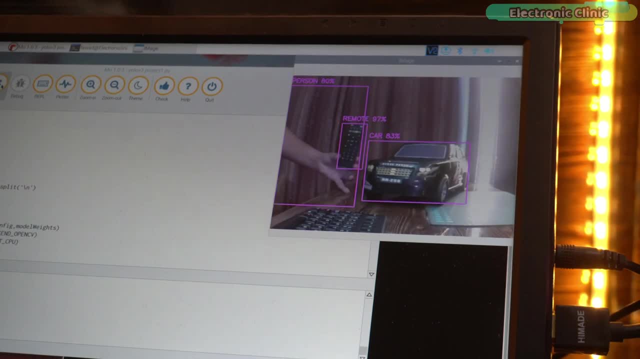 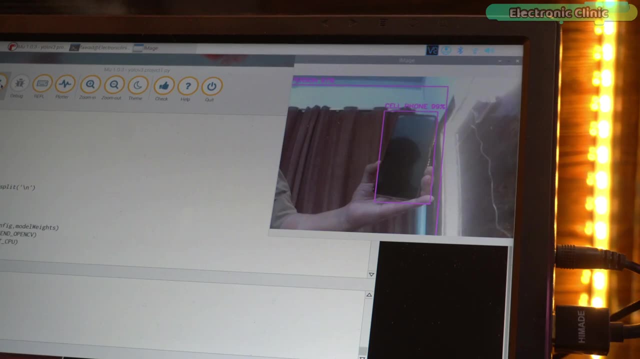 Raspberry Pi 4 is perfectly detecting all the objects, but it's really slow, So Raspberry Pi 4 isn't good for image processing, Although the 8GB variant of the Raspberry Pi 4 is quite popular- you can even play games with it- 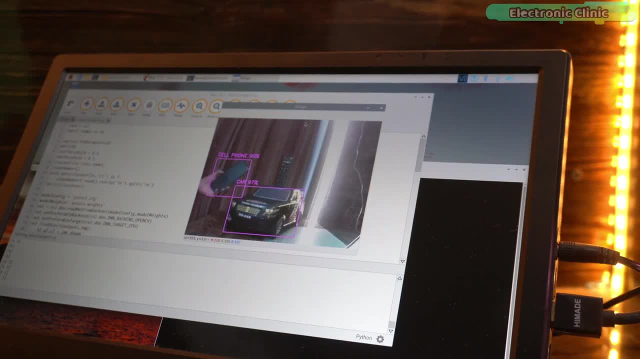 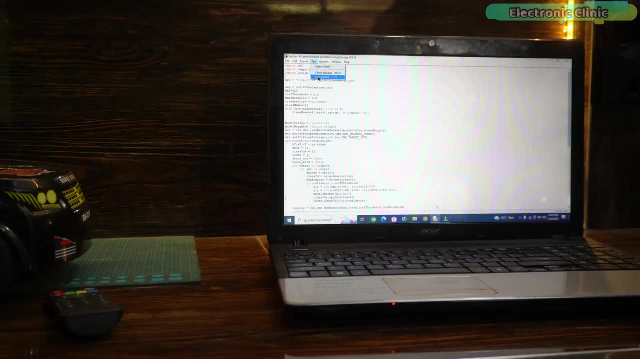 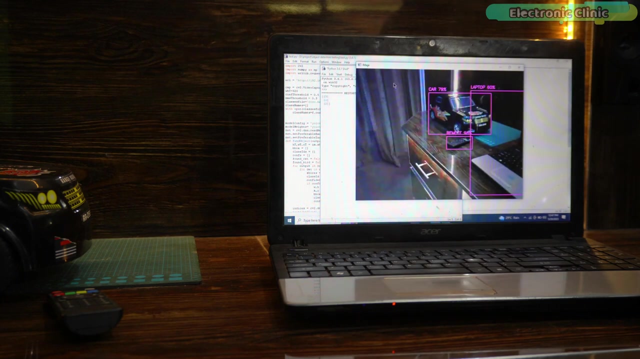 But when it comes to high-end image processing, it fails unless you add some kind of external hardware to it. Next, I am going to test this using Core i3 laptop, So let's go ahead and test this. It's working. It's working. 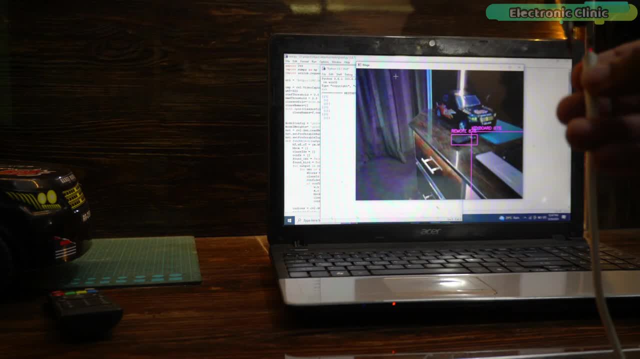 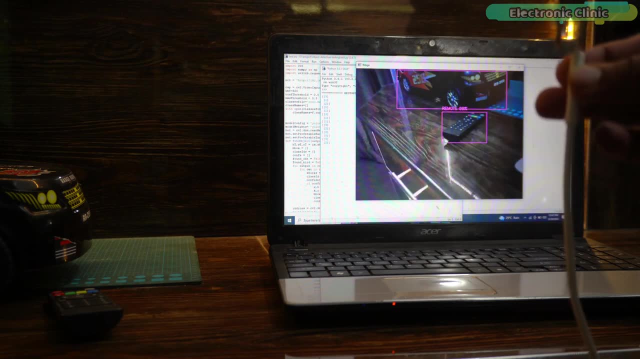 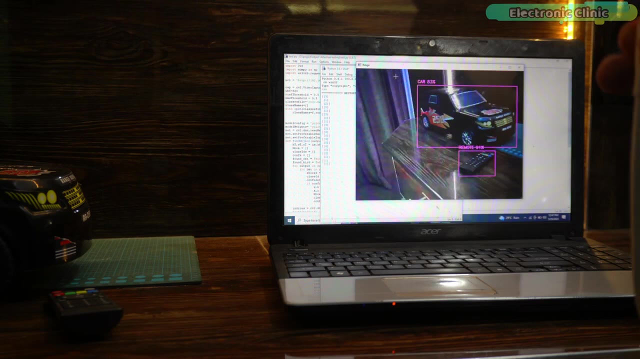 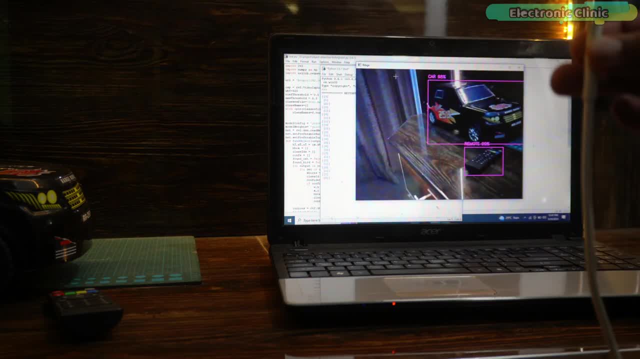 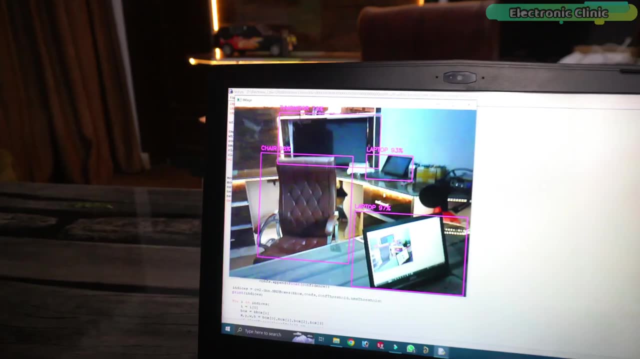 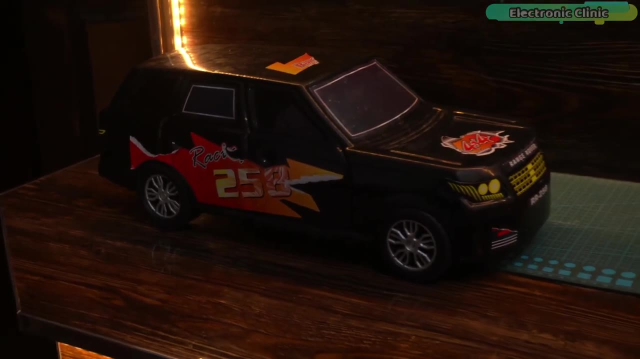 Anyway, if you have a Core i3 laptop, then this is what you can expect. Next I am going to test it on my MSI Intel Core i7 9th generation gaming laptop. Image processing on this machine is quite impressive, although it's not very fast. but 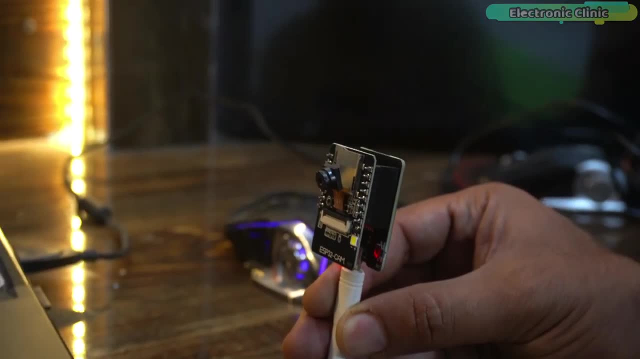 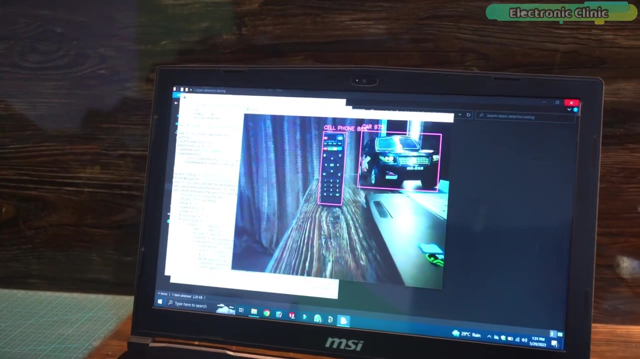 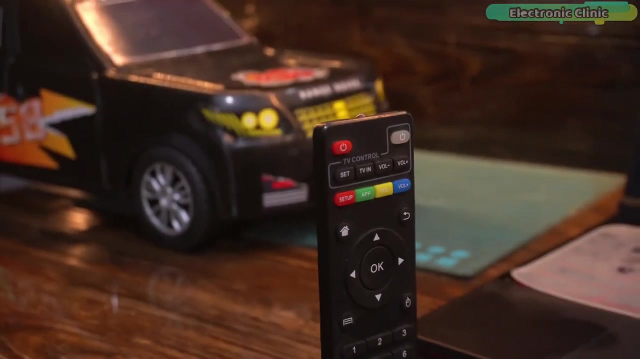 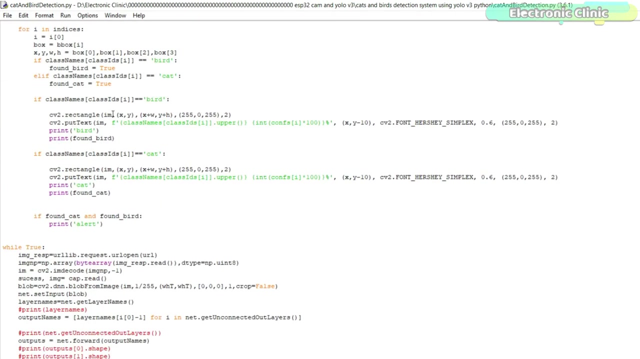 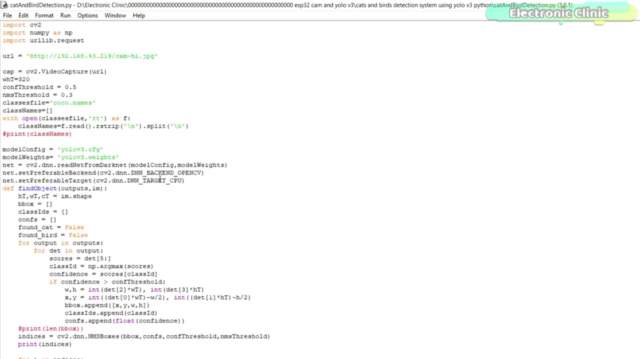 still, it's acceptable for me. I can use it in my future image processing based projects. Now let's check this final code, written only for the detection and identification of birds and cats. It will ignore all the other objects. For the line by line explanation, read my article available on electroniccliniccom.